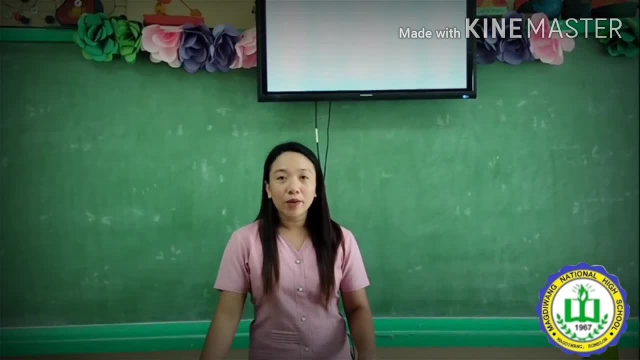 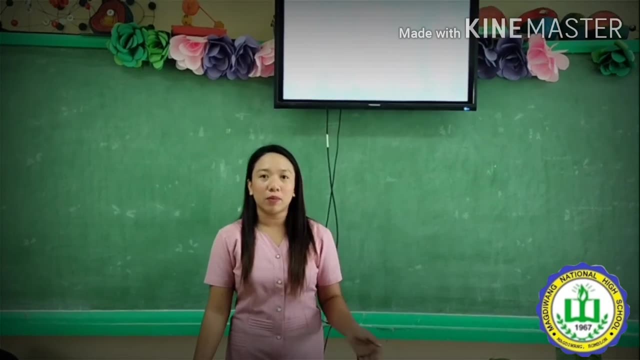 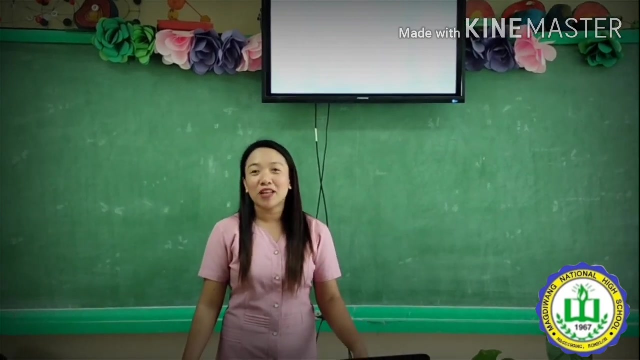 So I hope this video will help you. Anyway, our subject is physical science. It needs the teachers to discuss thoroughly about the topic, So this video will, I bet, help you understand more about it. But anyway, I will be using the Tagalog language so that we can all understand better, Especially for 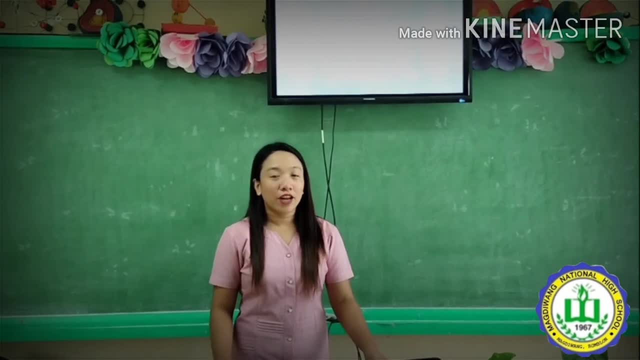 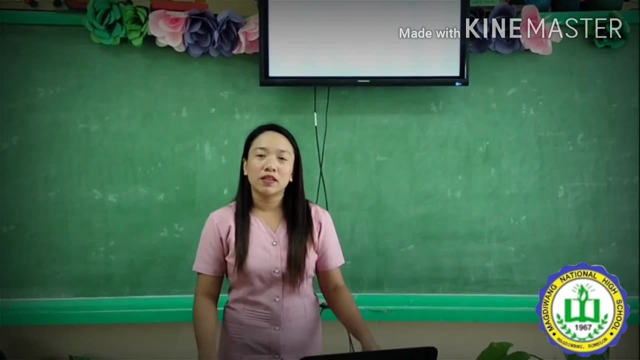 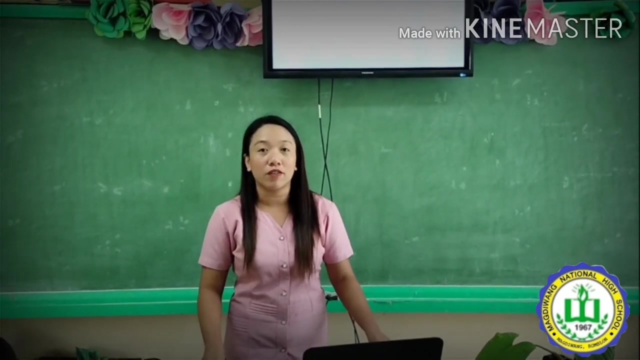 struggling students And for the information of everyone, our topic covers the competencies that was included in the ADM, or the alternative learning mode suggested by the curriculum experts of the DepEd. So please allow me to start. Have you also wondered what stars are made? 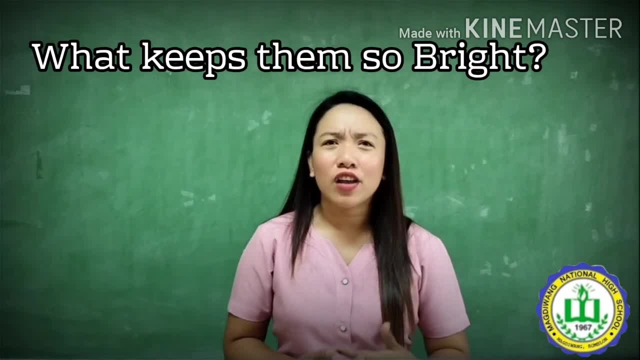 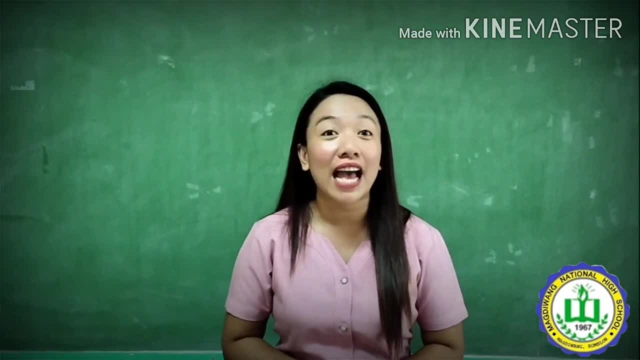 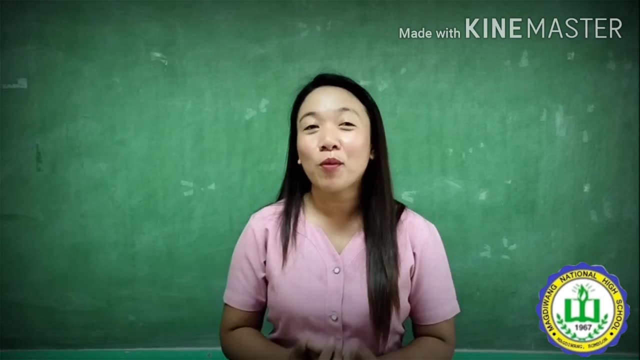 of What keeps them shining so bright? Are there also stars that do not spark? You might be asking the same questions since you were little that until now, you are still seeking answers for it. Well, this lesson will help you understand some of the important concepts about stars. 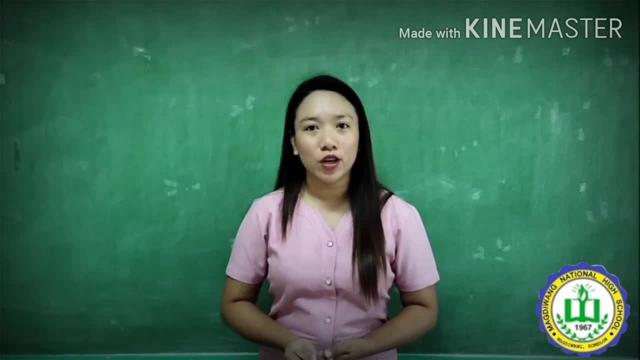 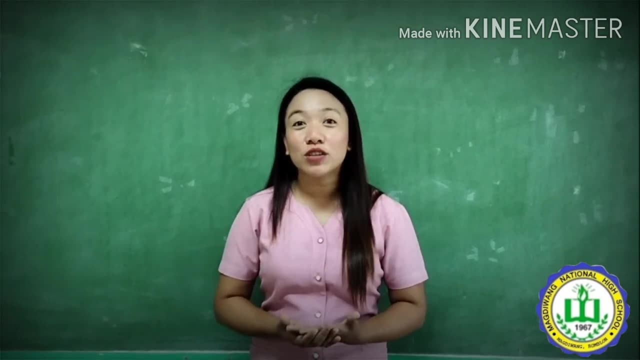 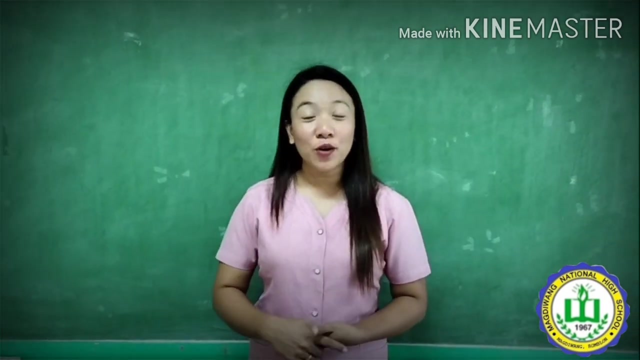 The world where we live today is just a small part of the universe. In your previous years, you have learned the different theories of the origin of the universe that eventually lead to the formation of solar systems, galaxies, stars and other heavenly bodies. So this lesson will focus on one of those wonderful things present in our universe. 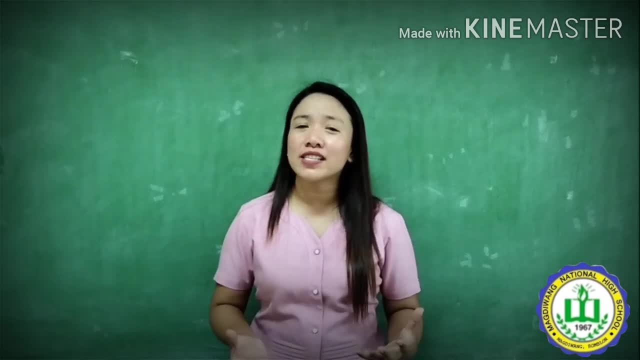 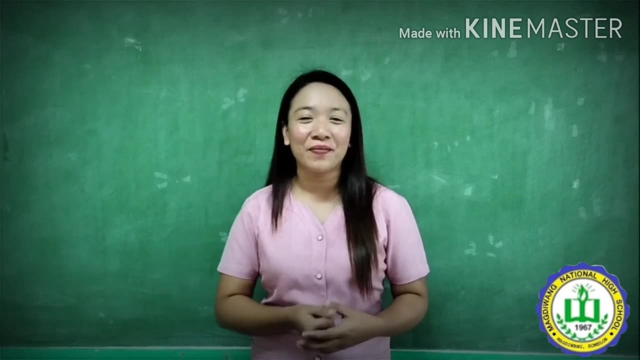 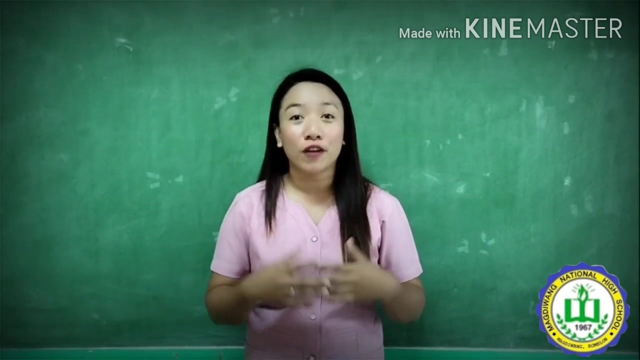 And, of course, the stars. Although stars are millions of light years from us, we can still see them in the night sky twinkling right. So let's find out how they emit light and how and what keeps them shining for a very long time. 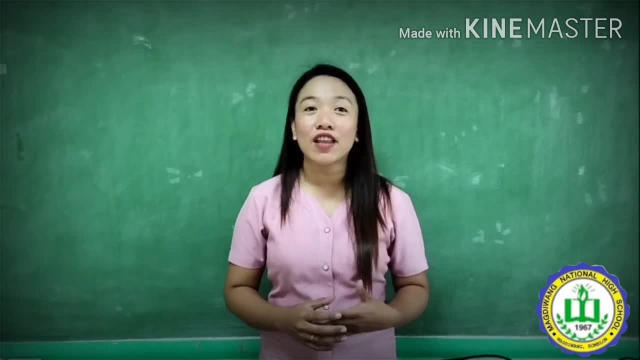 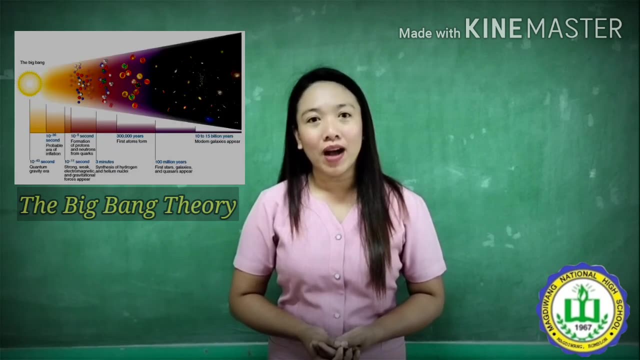 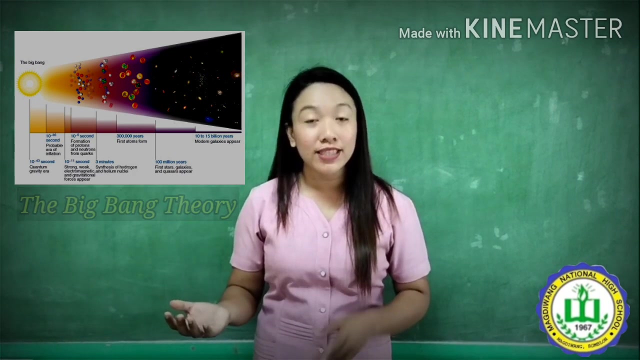 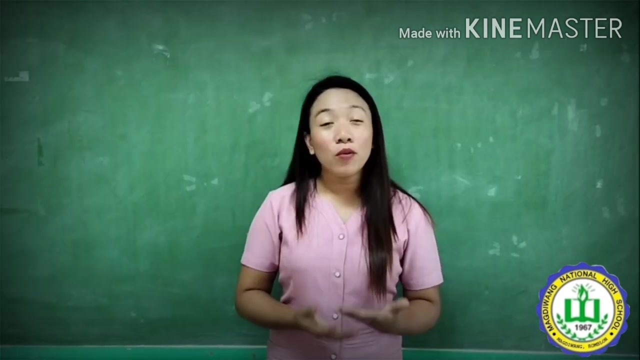 Scientists believe that the formation of the universe began through the explosion of primordial atom. that happened 13 billion years ago. It was known as the Big Bang. It became a theory that also explains the continuous expansion of the universe And, take note, it is the theory that most widely accepted because of its evidences Moving on right after. 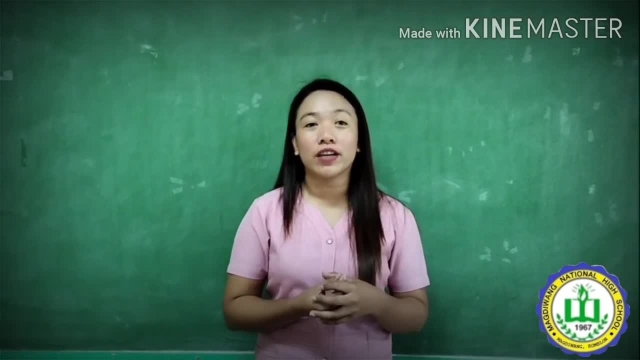 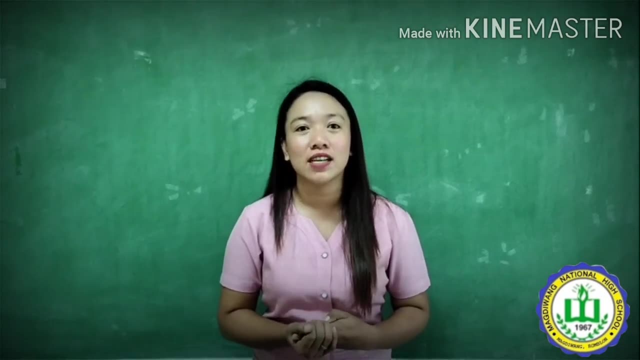 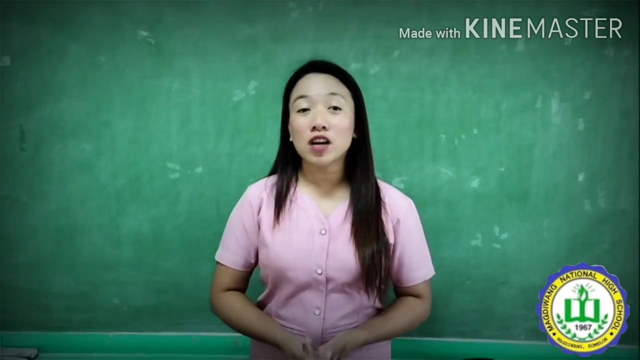 Big Bang, protons and neutrons combine together and form light elements like hydrogen and helium in the process of Big Bang nucleosynthesis. Other light elements, such as lithium and beryllium, were also found during this process. The first stars formed about 100 million years after Big Bang, and 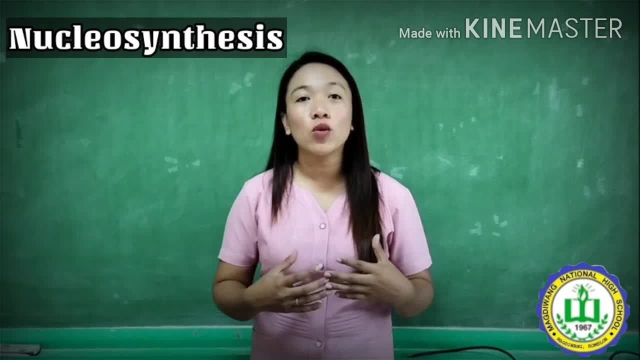 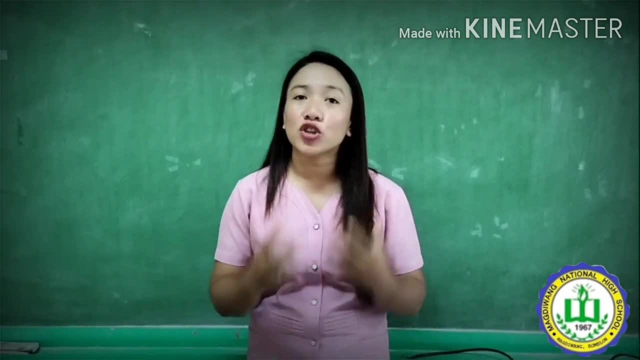 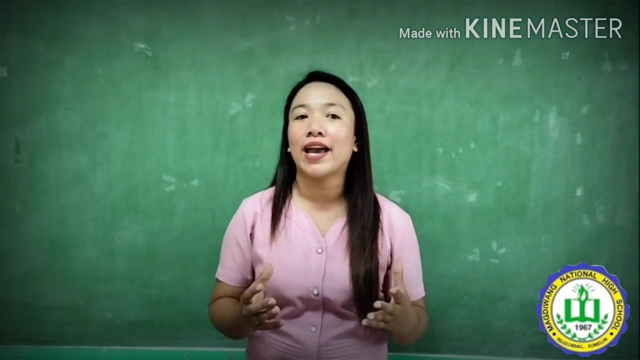 began a new type of nucleosynthesis. When we say nucleosynthesis, it is the process of forming or binding together. So the extreme temperatures and pressure in the core of the stars overcame the mutual repulsion of atomic nuclei and alloy nuclei to fuse together into heavier elements. 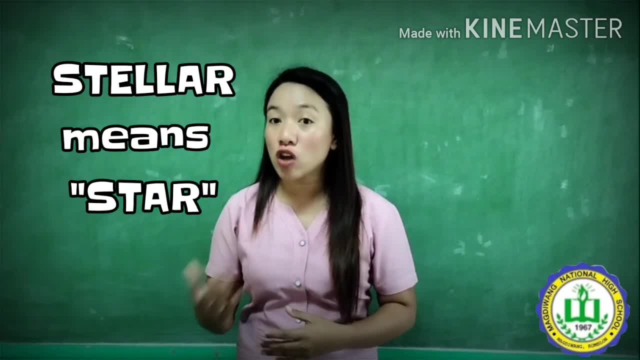 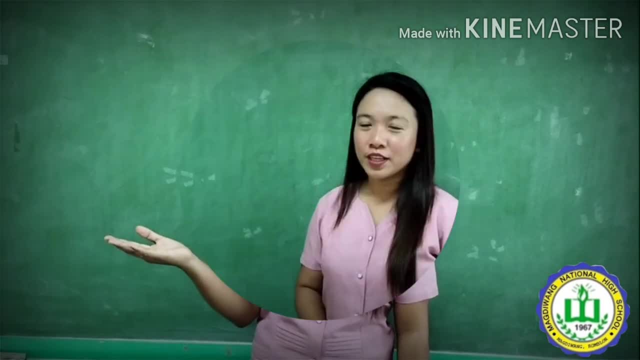 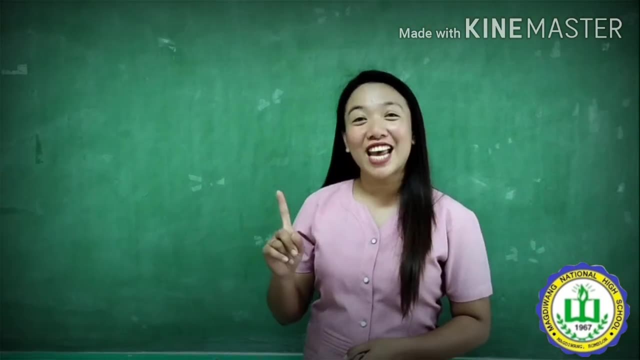 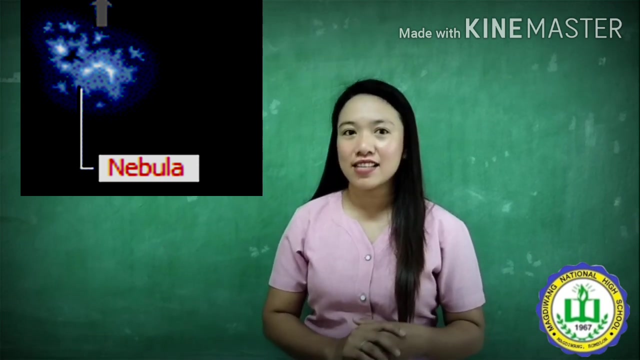 So the word stellar means star, and the formation of elements in the center of the star is called stellar nucleosynthesis. So this is the big picture of how the stars evolve. Let's explore them one by one. The first stage is the nebulas. Nebulas are clouds of interstellar gas and dust. 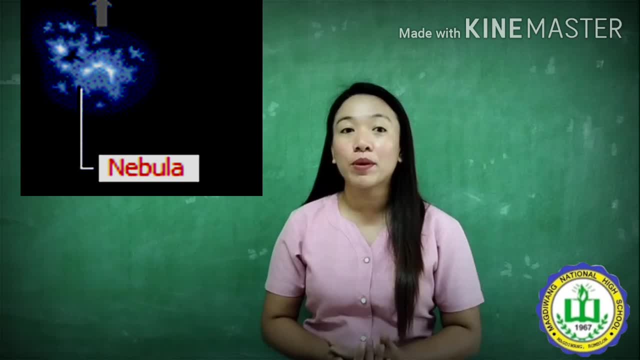 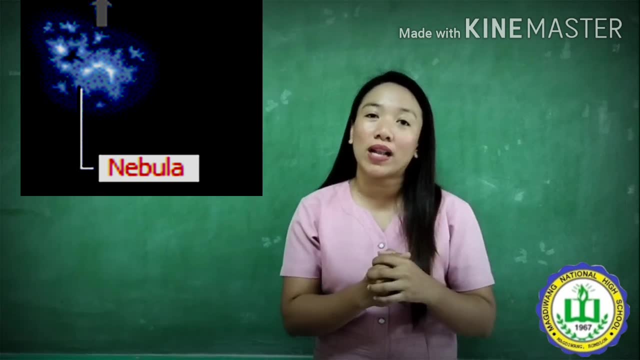 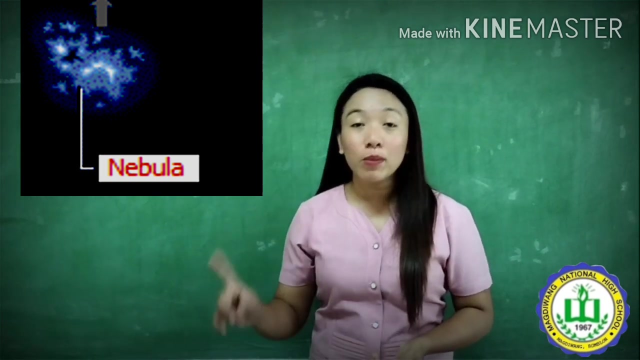 The gravitational attraction that material in a nebula has for itself. that can eventually make the nebula qualities. when we say qualities united into a denser object called a protostar, Always remember nebula is just a mere gas and dust. This is the first stage of nebulas. 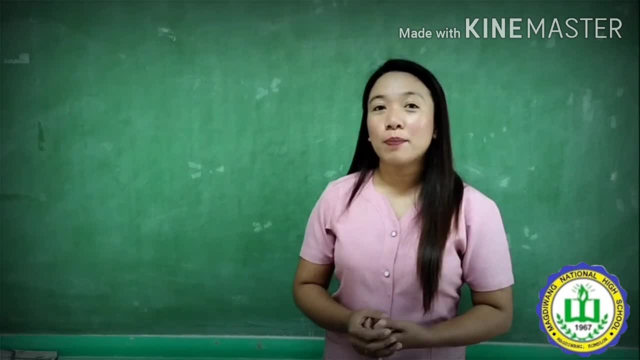 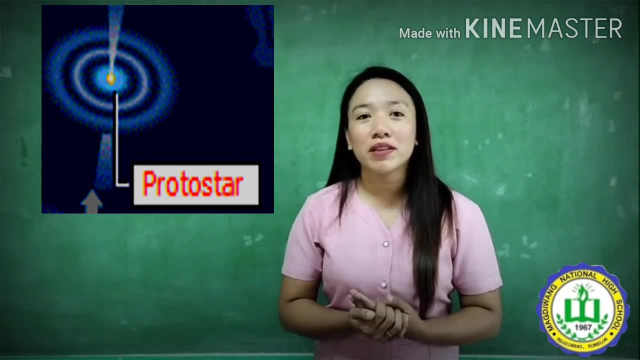 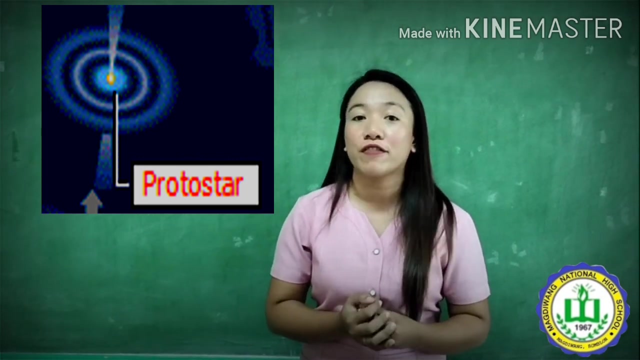 dusts. After a nebula, a protostar forms. when a dense region occurs in a cloud of interstellar material, The surrounding material is gravitationally attracted to this dense spot and condenses into a more compact form. As the material becomes more dense, it means pag lalo itong. 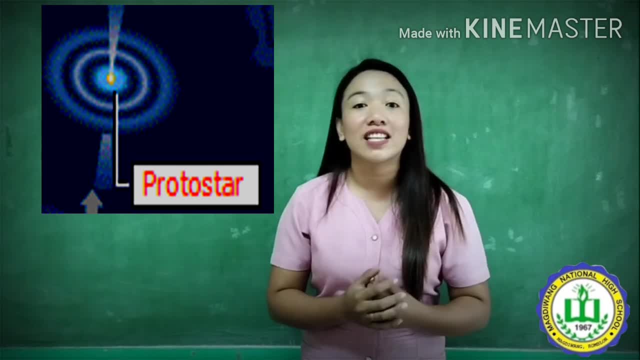 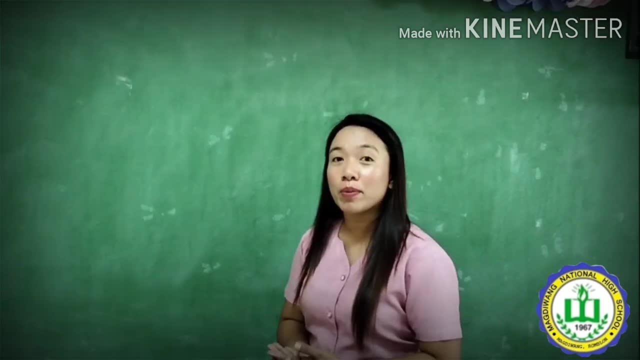 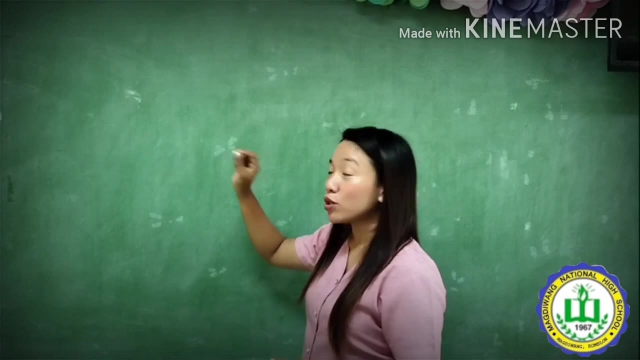 mas bumibigat, the pressure and temperature at the center of the protostar increases. So for you to easily memorize or remember concepts of the stellar evolution, let's have a mnemonic. So the first stage in stellar evolution is: N stands for the nebula. second, one is: P stands for protostar. So the third stage. a protostar became a star when its inner temperature reaches 10 million degrees celsius or 18 million degrees celsius. So it is a star when its inner temperature reaches 10 million degrees Fahrenheit. This high temperature. 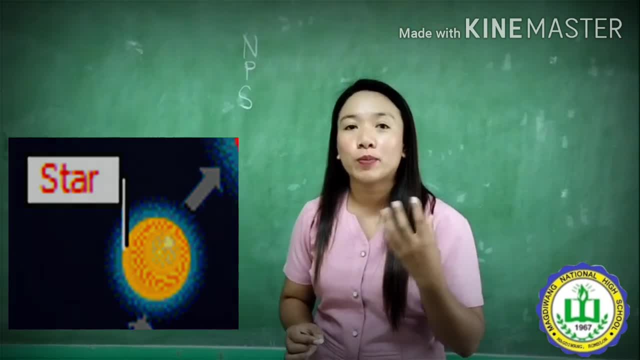 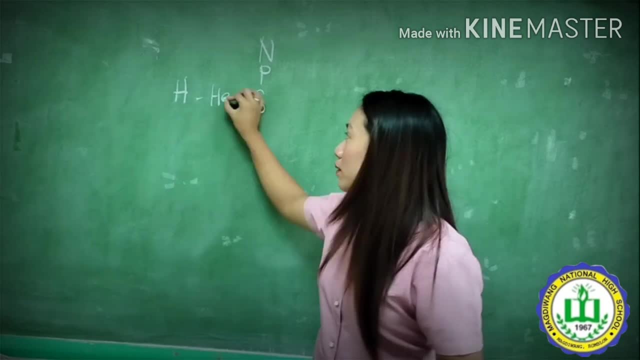 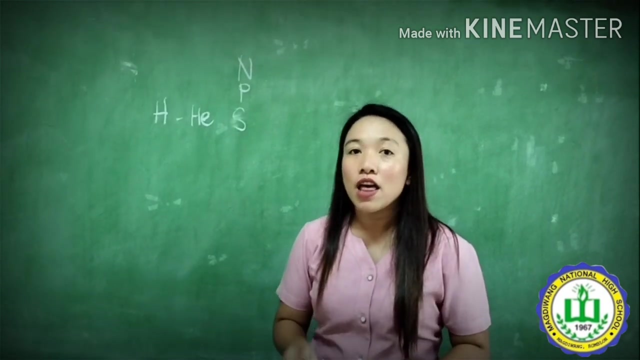 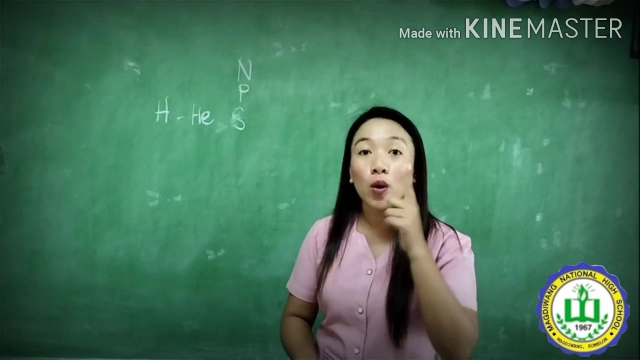 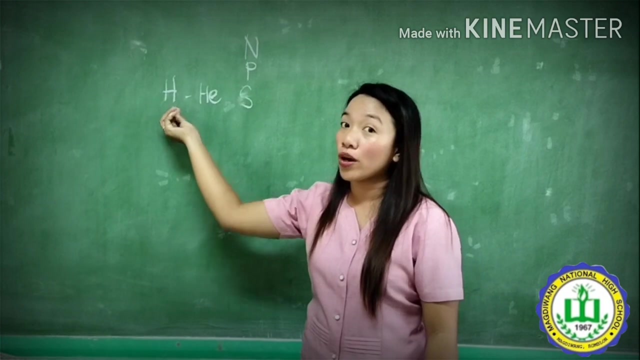 triggers a nuclear reaction in the core of the protostar, Hydrogen fused to form helium and releasing a tremendous amount of energy in the process. This energy fuels the star and radiates outward in the form of light and heat. The core of the star is none other than the light elements called helium or hydrogen. So a star evolves into a red giant, RNG, when its hydrogen fuel begins to run out. So when it consumes its fuel, the hydrogen red giant forms. The core of the star shrinks as it nears the end of its hydrogen. but the outer layer of the star also shrinks as it nears. 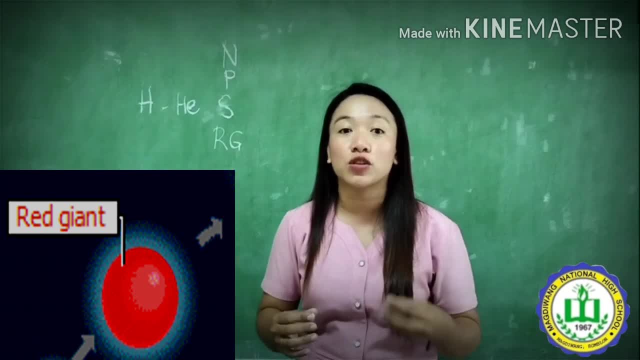 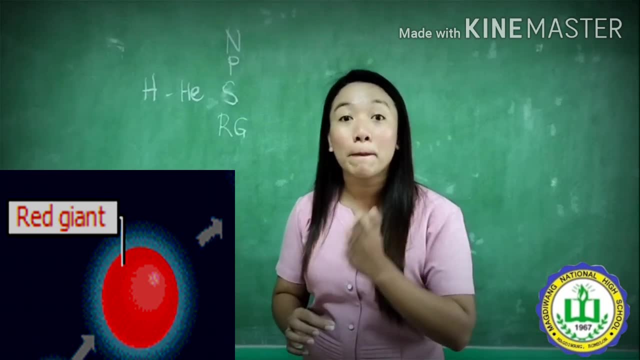 the end of its hydrogen. but the outer layer of the star also shrinks as it nears the end of its hydrogen. but the outer layer of the star also expands as the star begins to burn its core. A red giant can grow to be 100 to 1000 times bigger in diameter than the Sun. 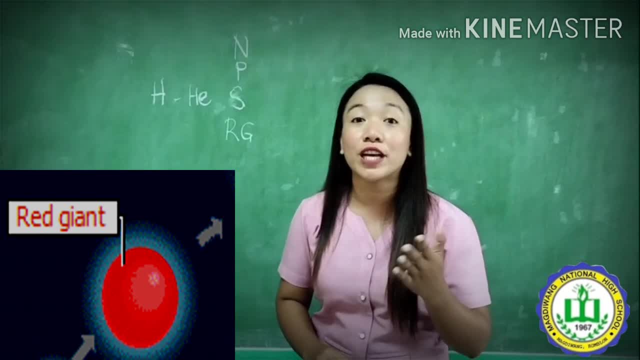 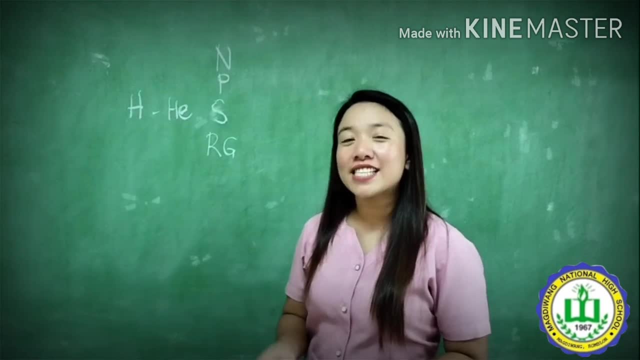 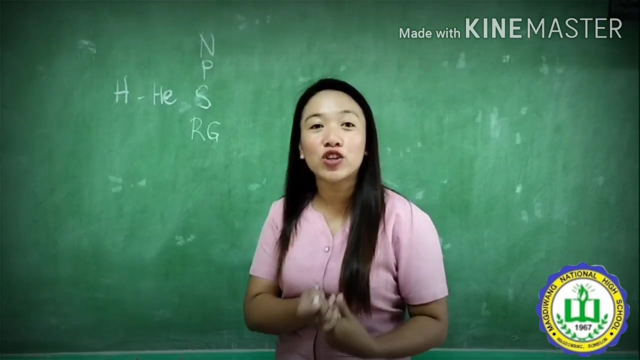 imagine that, but its surface is relatively cool, making it glow with a red color instead of blue or white. For the next stage, when a very massive star goes through a second expansion, after exhausting their hydrogen fuel, they become supergiants or SG. okay. Supergiants form when helium atoms in the core of massive stars, red giants or massive red giants fuse to form carbon. So when the helium fuses with other elements that forms carbon supergiants was produced, These nuclear reactions release a second wave of energy and cause the red giant to expand. 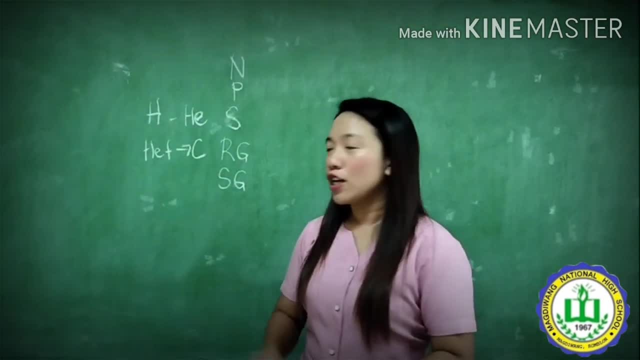 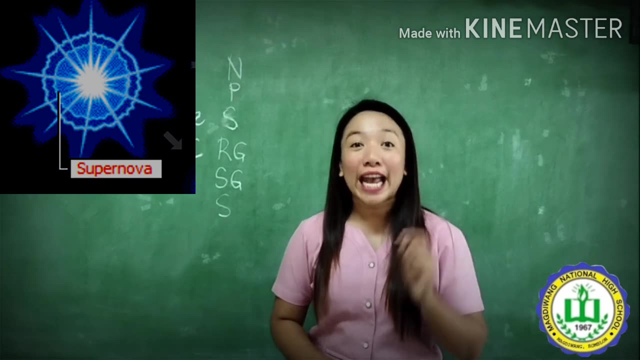 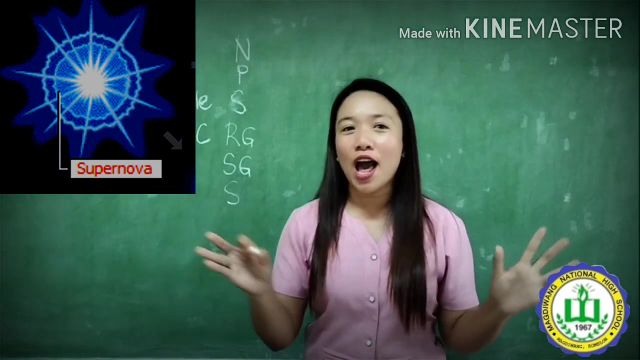 into supergiant Moving on. supernova. stand for. X occur when very massive stars, more than 8 times the mass of the sun, use up their fuel and collapse boom under their own weight. The collapse leads to an explosion that sends a shockwave. 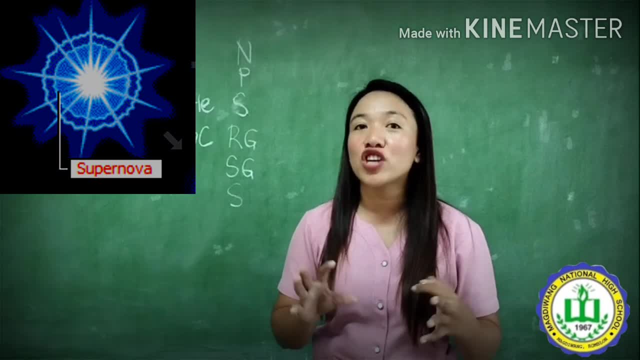 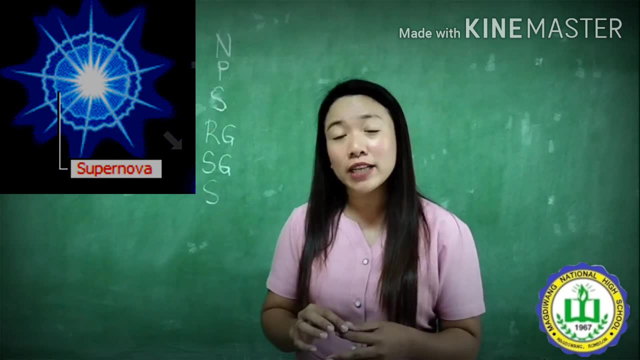 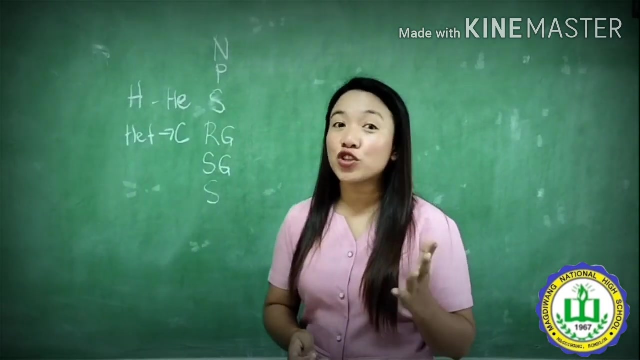 A shockwave through space which is followed by a shell of material from the star's atmosphere. The supernova may completely destroy the star or it may leave the core of the star intact, So it depends upon the process itself. When an extremely massive star supernovas the gravitational pull within their remaining 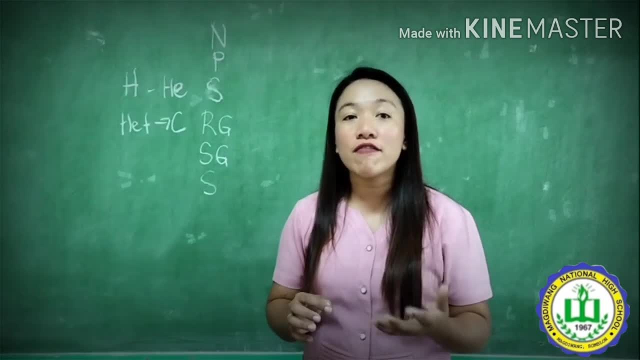 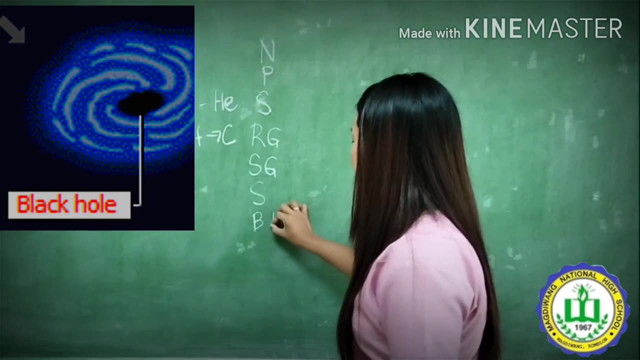 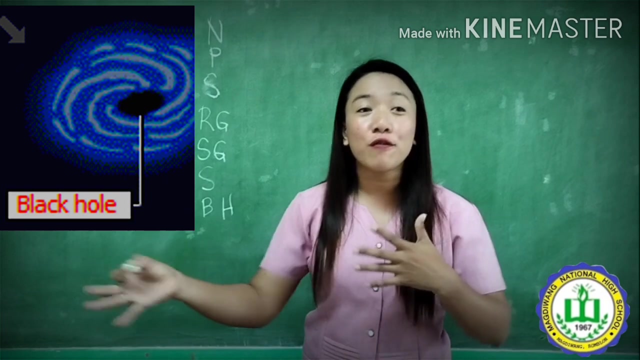 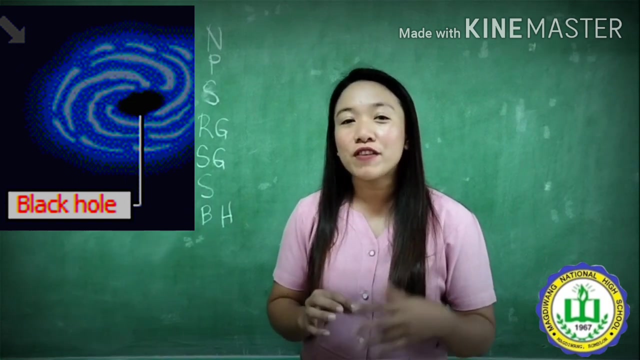 core may be strong enough to cause even neutrons to collapse. The core condenses into neutrons. The core condenses into neutrons. What do supernova form? Supernova, basically, would look like a picture in the distance. This is important too if you want to capture themates of a single citizen in behavior off. 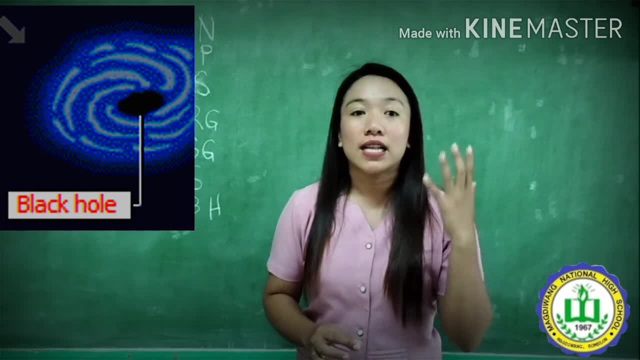 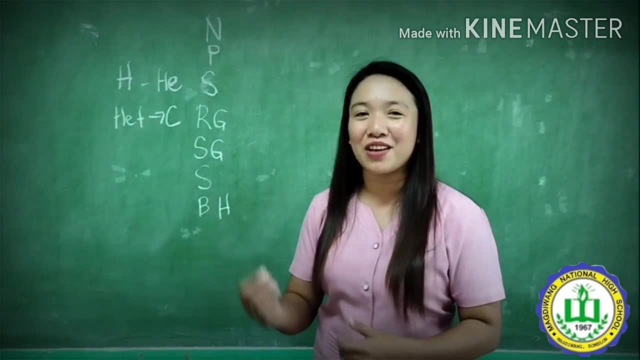 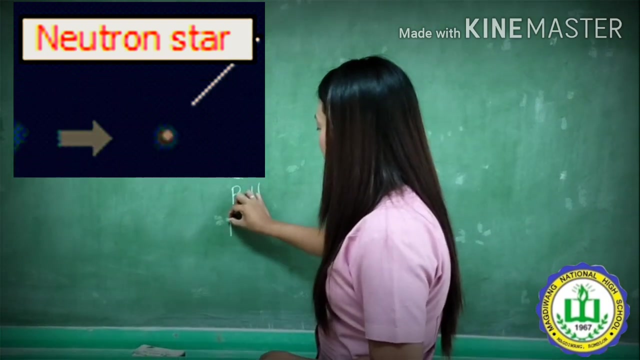 a star. it would almost face the sun's right arm when that happens, So that's why it is called a black hole. It forms a black hole. This is an object so dense and eventually the so-called the corpse of the star, the neutron star, it forms. 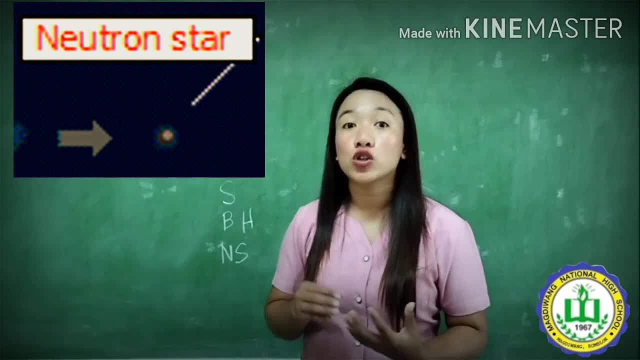 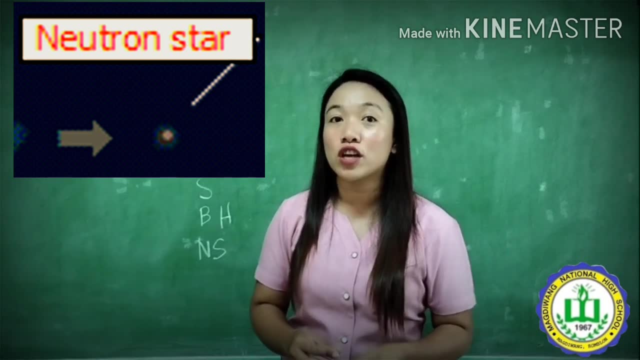 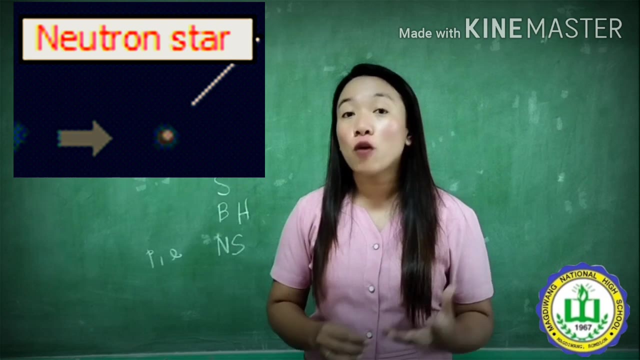 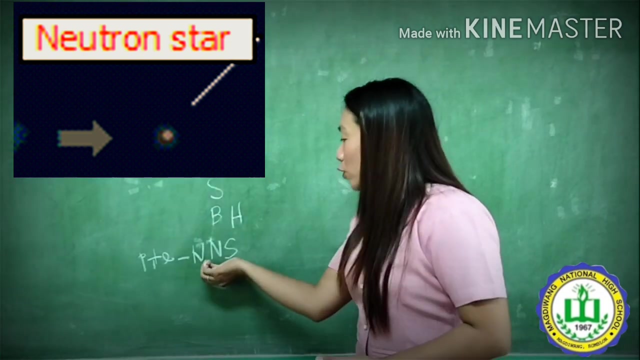 from the core of the star that has undergone supernova. the atoms in the star condenses and collapse until two particles that compose atoms, the protons and electrons, fuse to form neutron. when protons and neutrons are fused and they form neutron, neutron star was being produced. the star is no longer composed. of complete atoms, only neutron. so that is why it is called neutron star. so, aside from this way or you will see something like this is another reason why the proton is gäller. kaya nga tawag sya neutron star. so aside from this way or 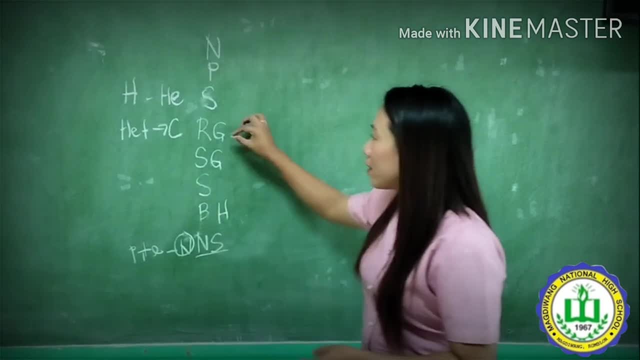 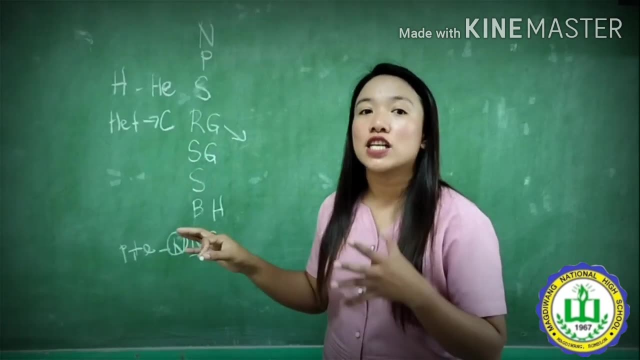 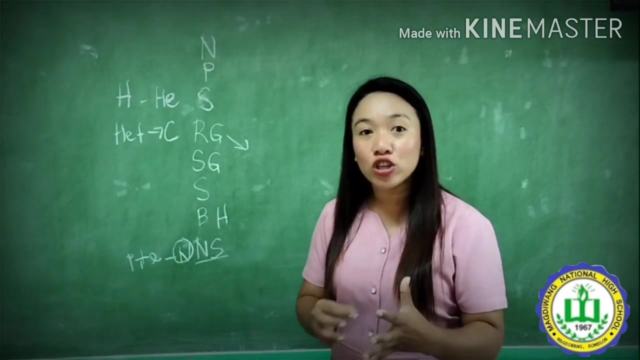 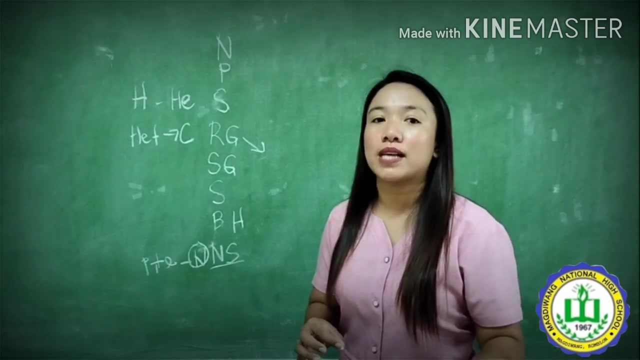 this stage. uh, there is also another stage, when star can also undergo so, when a red giant that is six to eight times more massive than the sun run outs again the fuel- no one had a shining hydrogen- the star becomes unstable and collapses it. it collapsed, and under its own weight. 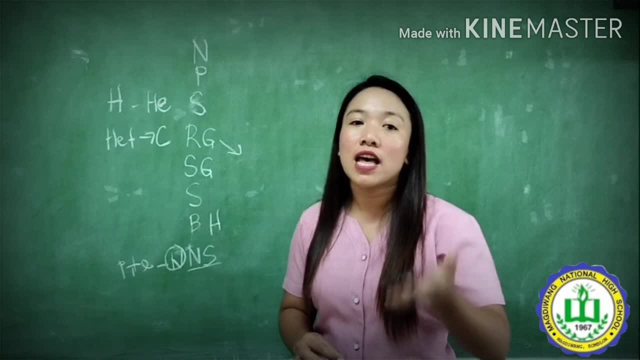 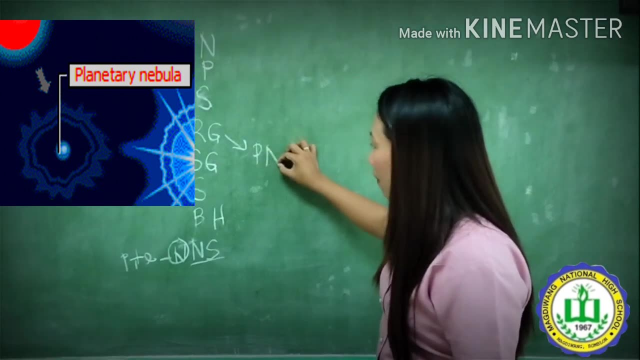 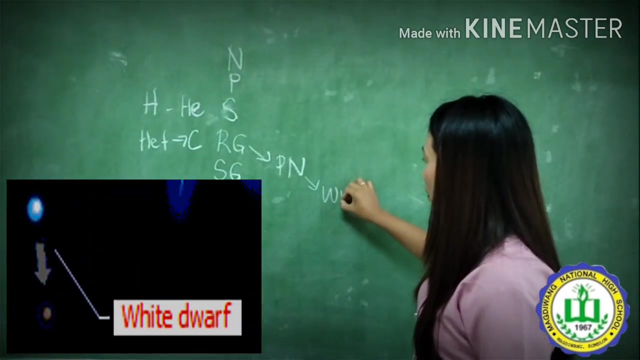 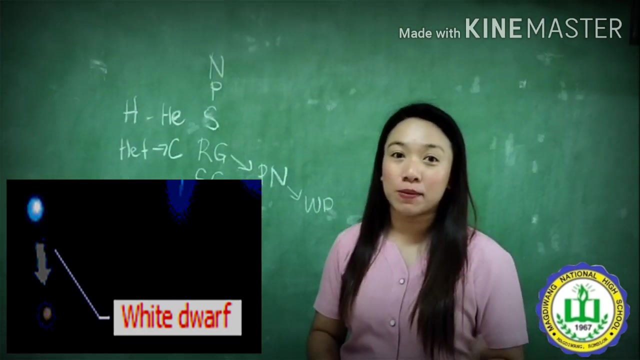 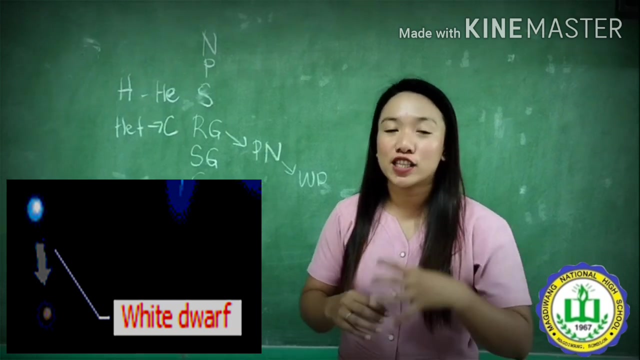 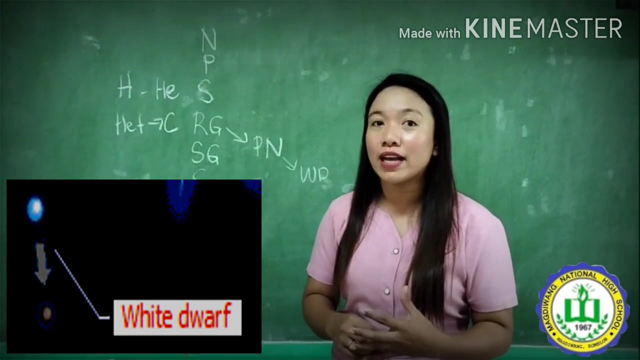 injecting its outer layers into space. this hollow ejected space or gas and dust forms the planetary nebula, now a white dwarf. white dwarf forms when a red giant use up its fuel and collapses such a star, extremely compact, and continues to glow because of energy drop in its core. white dwarf can be as small as earth, yet contained as much- 70 percent- of the mass of the sun. 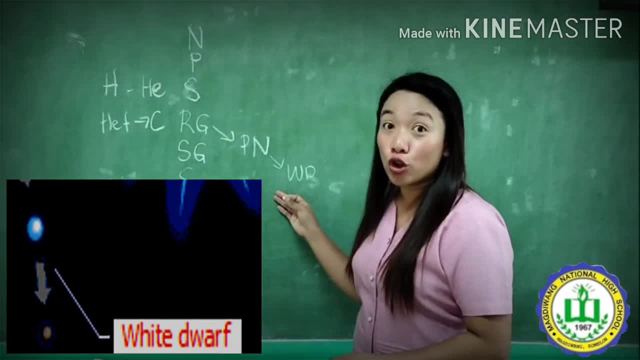 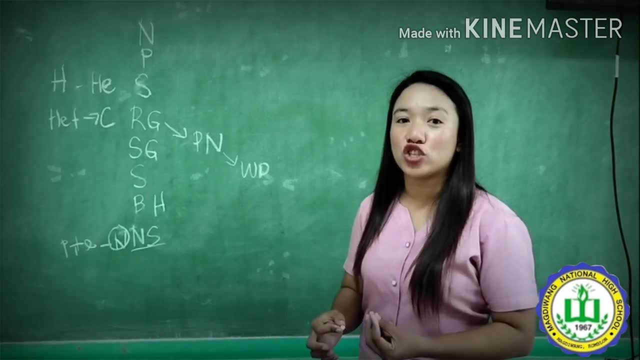 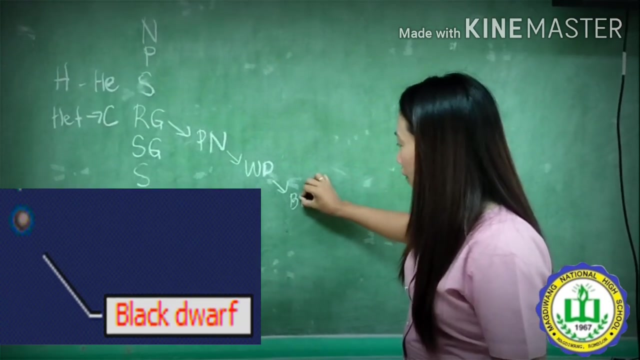 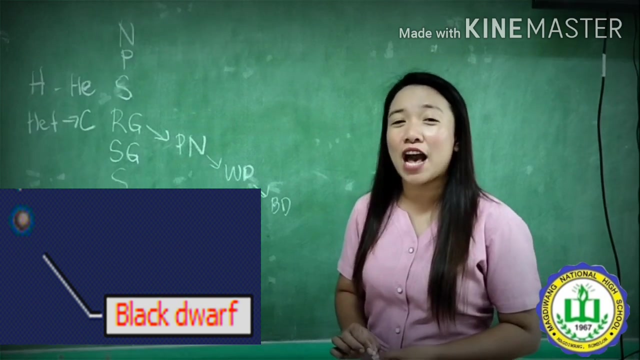 remember white dwarf still glows now when a white dwarf eventually releases all its truck energy and cools off, but it became black dwarf. black dwarfs are much more. black dwarfs are much more massive than planets, but they are too cold enough to give off life, meaning they are not sparkling or